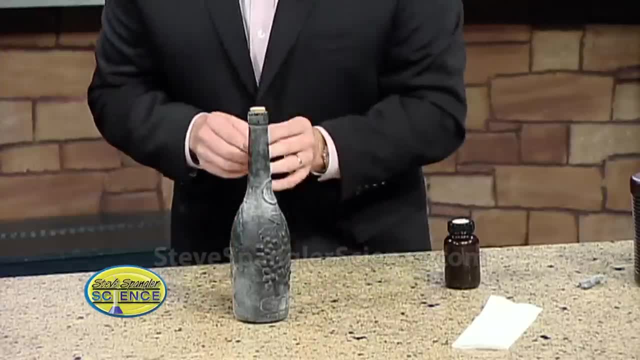 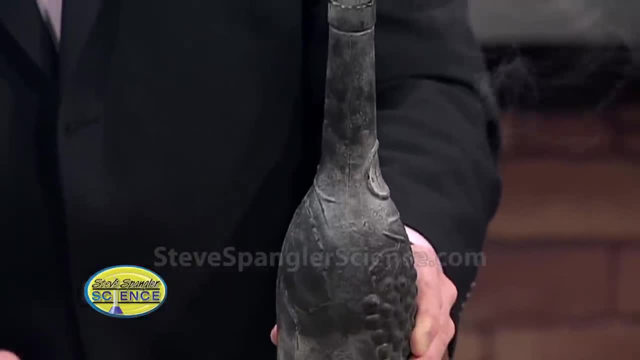 I know, Get out, I will bring the prod. No, All right, Oh, we have to uncap it because it is a lazy genie. So here's old great genie. Let's see. Oh, oh great. Oh my gosh, Would you look at how? 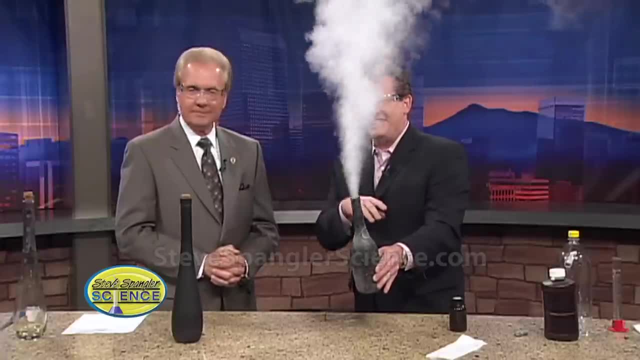 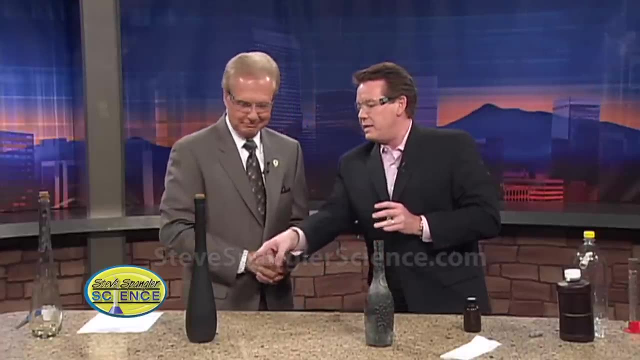 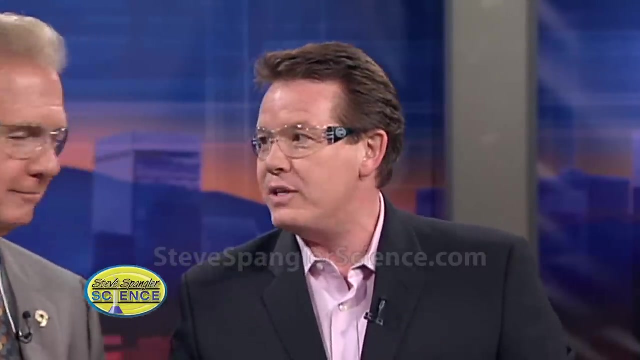 great. Wow. Smells a lot like a genie too. Bottles getting warm, Mark. viewers have said: I tell you the secret too quickly, So it is your. I set up one for you. There's a genie inside. Honestly, there's not chemicals, So it's just a genie inside there. So you open it up and then I'm gonna let you guess. 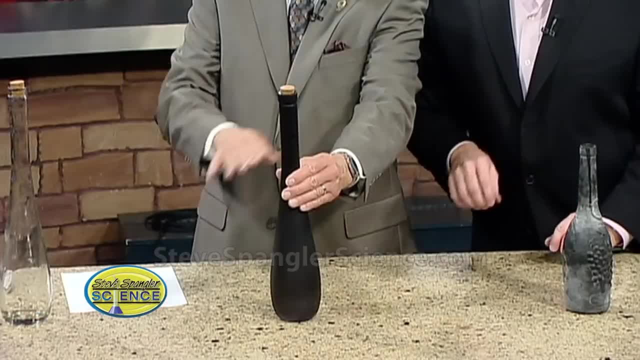 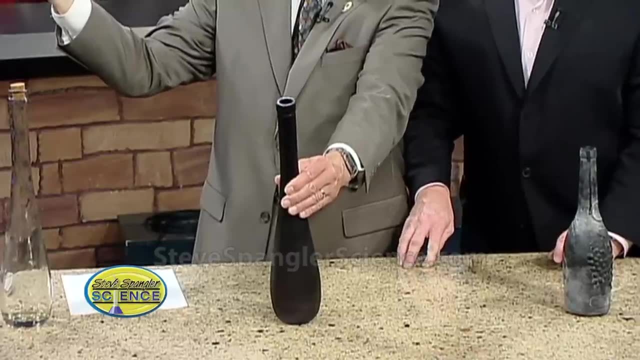 how it works. Fair enough, All right, This one. Oh great genie. Oh great genie. Very good, Please exit The bottle. Toy Story made one hundred and thirty million, One hundred and thirty billion this weekend, Somehow, And nothing. Oh, the genie had to be rustled just a little bit. Oh yeah, Maybe we 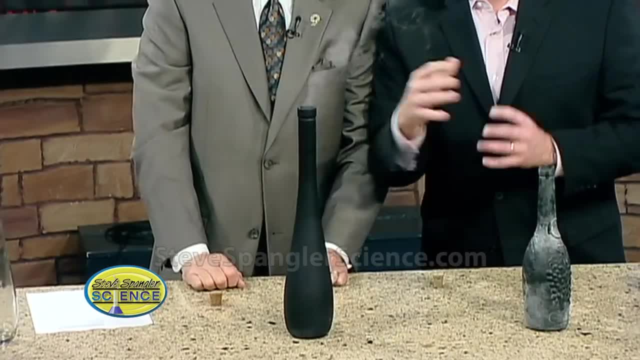 got My genie, My genie, My genie is rusting. Oh, You did not grant you as many wishes. Oh, there you go. There it is though. Oh, how cool, Isn't that? very, very pretty. That is so cool, So a special. 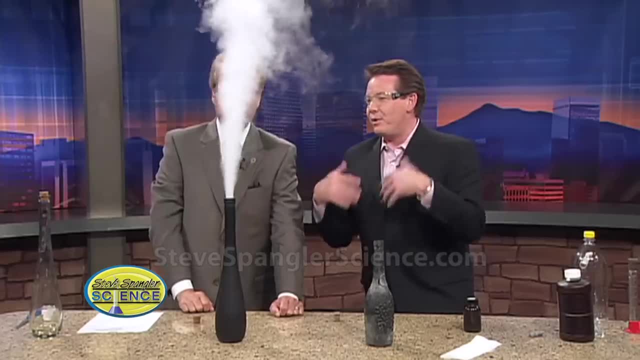 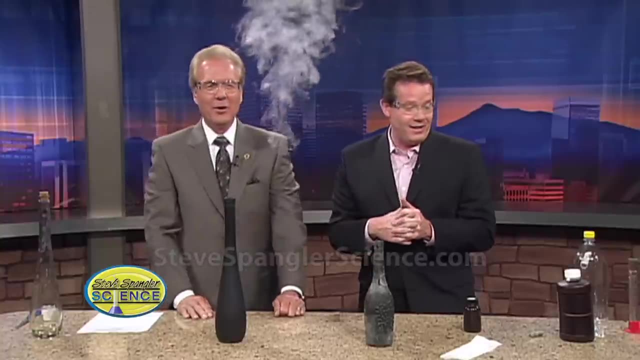 effect artist will will use something like that. Honestly, the burning sensation in the lungs goes away after a while. So that's, It's a little pungent, That's a little. Yeah, genie needs to take a shower, That's all right. So so I'll give you a little secret. There is a chemical. 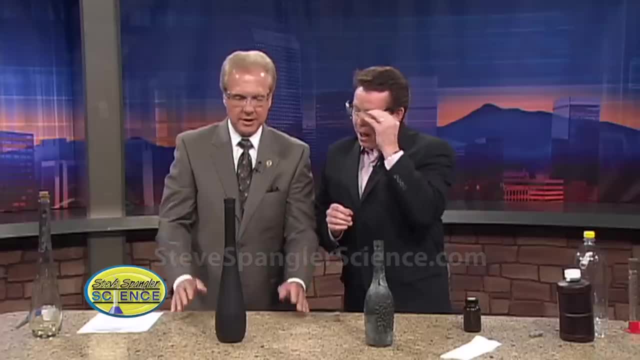 down inside Any idea what that is? It's obviously not not nitrogen, or or No, because it's warm, Yeah, So the viewers can't really, And you'll be able to see it here in just a second. Take a look at this. 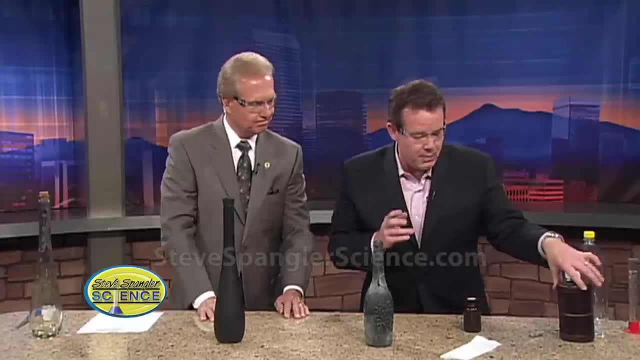 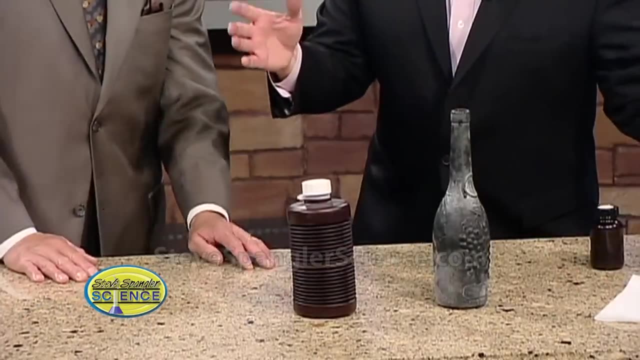 Is it sulfuric acid? No, because it'd be a little too dangerous. This is, But it's not like this isn't dangerous. Mom used to use something like hydrogen peroxide. Hydrogen peroxide- Right, So it's three percent. So you go to the store and you get that and it bubbles on your skin. It means it's. 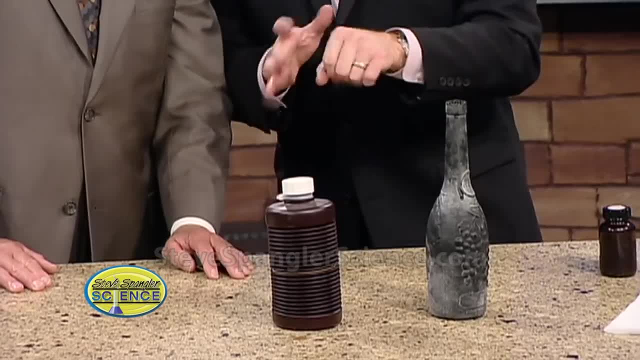 releasing oxygen. Well, this is thirty percent, So it's. And so you'd get burns on your skin if you even touch it. So you have to be very, very careful. Let me show you how we put the whole thing together. All right, All right. So if you bring over the 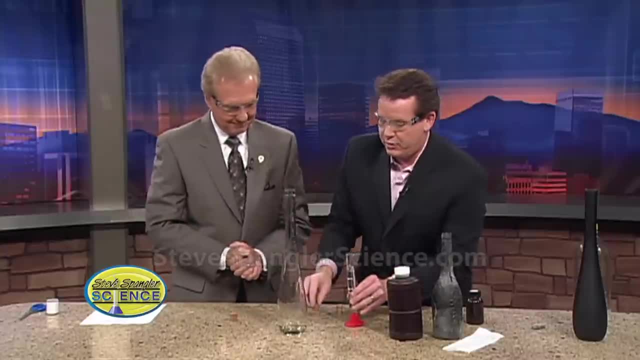 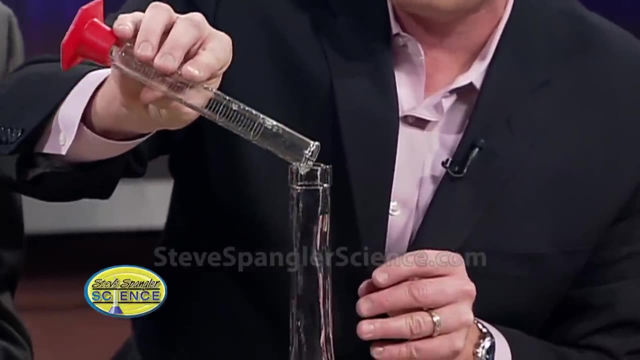 clear bottle. we'll show the viewers how we do it. So, first of all, we're using the 30 percent hydrogen peroxide and we've got to release the oxygen from there, And so we want that and we're going to have a little bit of that steam or that vapor that's going to come off as well. So there's.